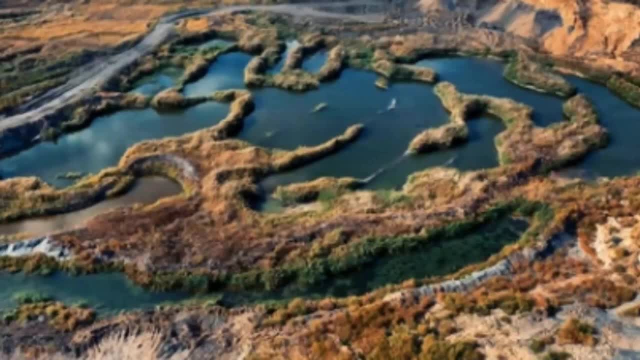 What is environmental geology? Environmental geology is a branch of geology that studies the interactions between humans and the environment with a focus on understanding how geological processes and natural resources impact the Earth's ecosystems and the human populations that rely on them. It involves the application of geological principles and techniques to identify and mitigate the environmental impacts of human activities. Environmental geology plays an important role in addressing global environmental challenges such as climate change, pollution, land-use change, and natural resource depletion. It provides the scientific basis for understanding the processes that shape the Earth's surface, the distribution of natural resources, and the impact of human activities on the environment. 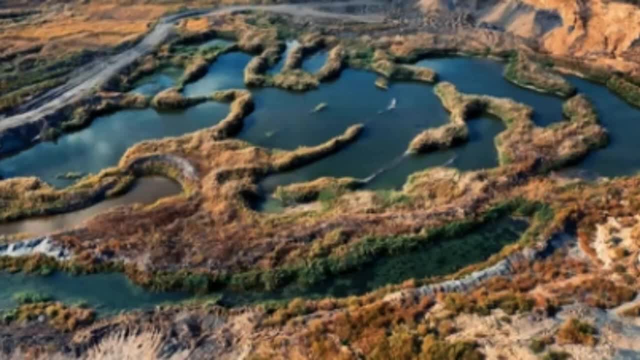 One of the key areas of environmental geology is the study of natural hazard systems and the impact of human activities on the environment. 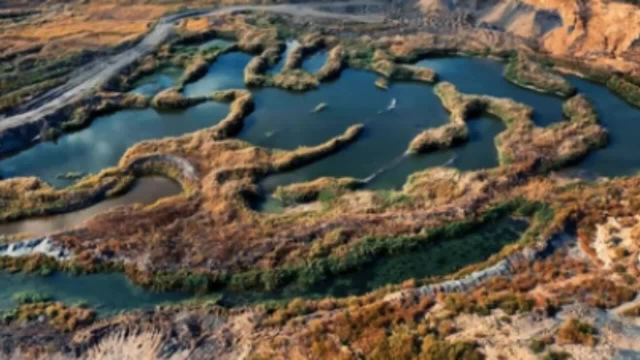 Such as earthquakes, landslides, volcanic eruptions, and floods. By understanding the causes and mechanisms of these hazards, environmental geologists can help mitigate their impacts by identifying areas at risk and developing strategies to minimize their 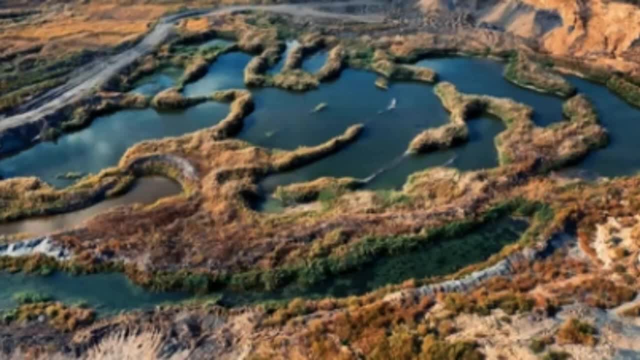 effects on human populations and infrastructure. Another important aspect of environmental geology is the assessment and management of natural resources such as water, minerals, and energy. 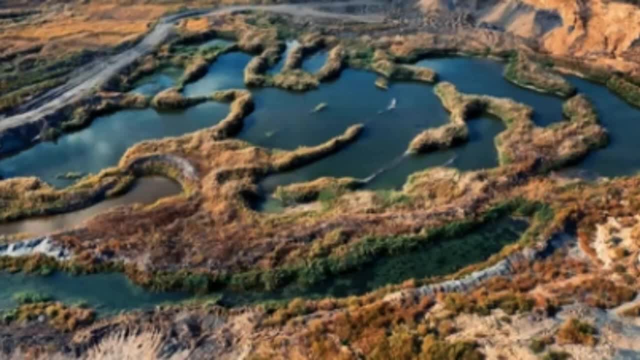 Environmental geologists use their understanding of the Earth's processes to identify and evaluate potential sources of these resources and to develop sustainable management strategies that 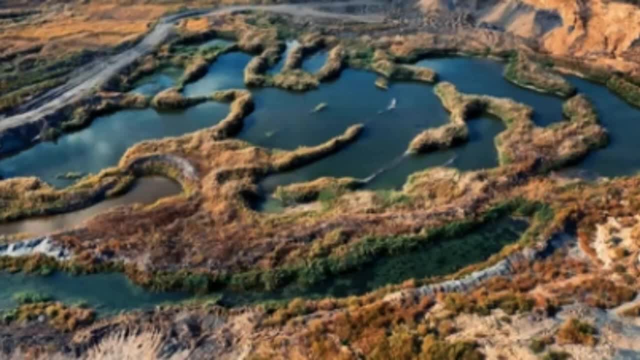 minimize their impact on the environment. Environmental geology also plays a critical role in understanding the impact of human activities on the environment. 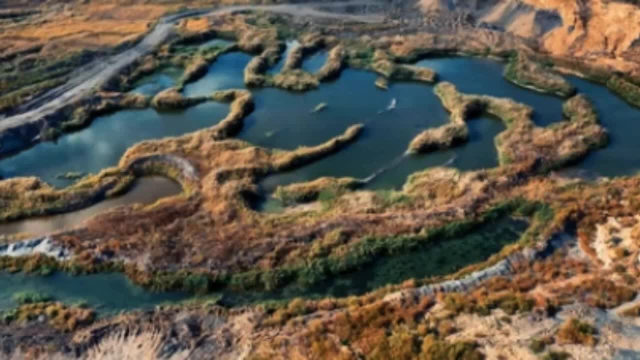 By studying the interactions between humans and the environment, environmental geologists can identify the environmental impacts of human activities on the environment and the environment. Environmental geology also plays a critical role in understanding the environmental impacts of activities such as mining, land use changes, and pollution. This information can then be used to develop strategies for mitigating these impacts and promoting sustainable development. 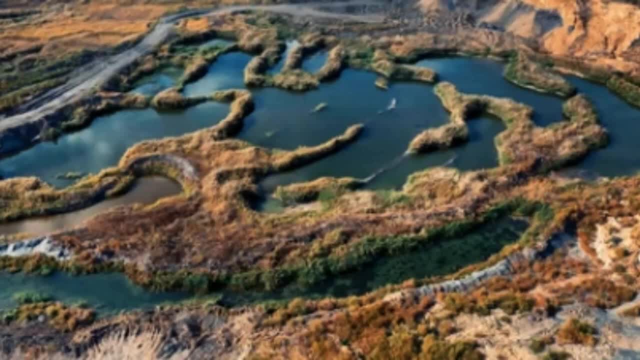 In recent years, environmental geology has become increasingly important as the world faces a range of environmental challenges, including climate change, pollution, and natural resource depletion. By applying the principles of environmental geology, scientists and policymakers can work together to develop strategies that promote sustainable development and protect the Earth's ecosystems and natural resources for future generations. 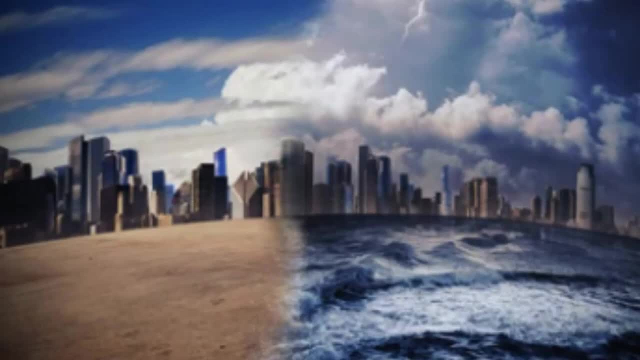 What are the fields related to Environmental geology? Environmental geology is a multidisciplinary field that draws on a variety of related areas to address 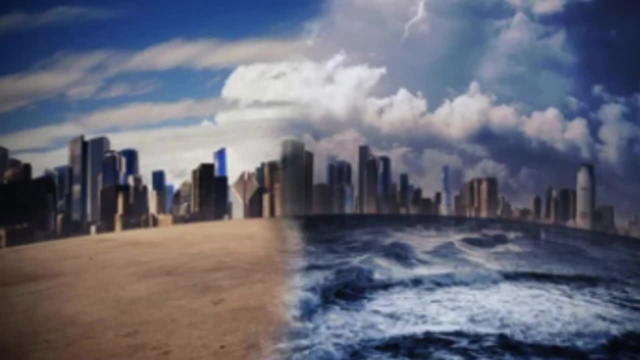 complex environmental challenges. Some of the related areas of study include. 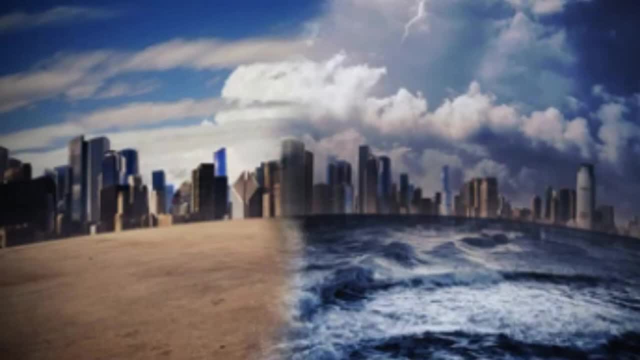 Hydrology Hydrology is the study of water and its movement in the Earth's system. 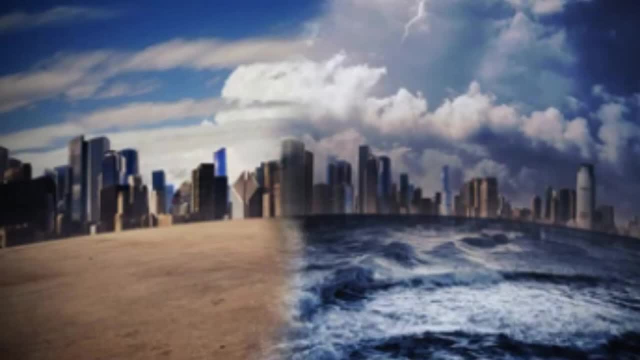 Environmental geologists work closely with hydrologists to understand the distribution of water resources and how human activities impact water quality and availability. 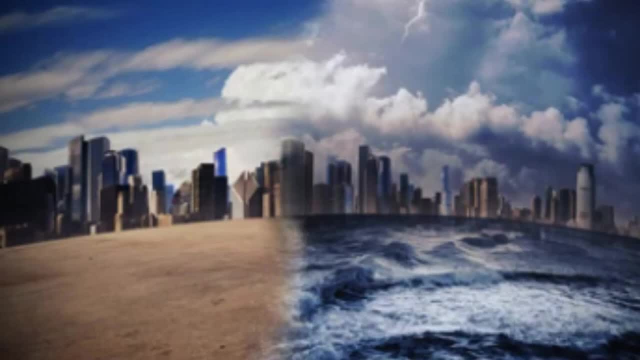 Geomorphology Geomorphology is the study of the physical features of the Earth's surface and how they are formed. 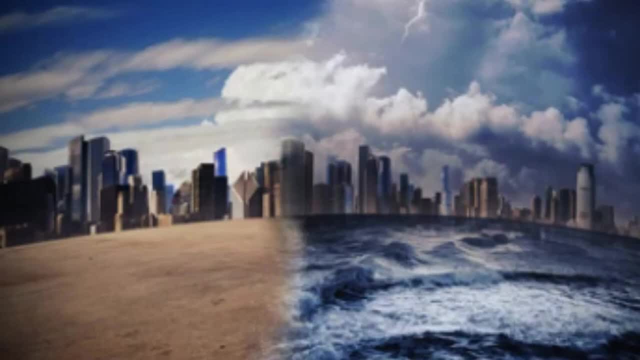 Environmental geologists draw on geomorphology to understand how natural processes such as erosion, weathering, and deposition shape the landscape and how human activities can impact these processes. Soil Science 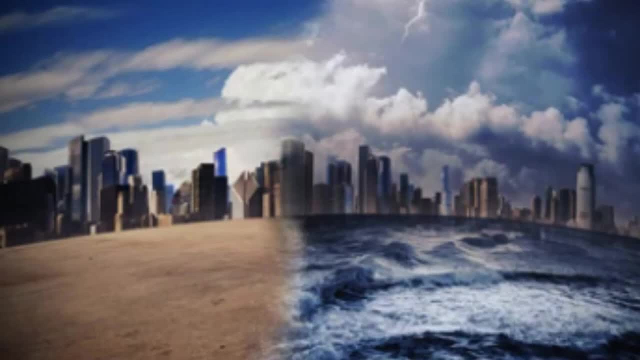 Soil science is the study of the composition, structure, and properties of soils. 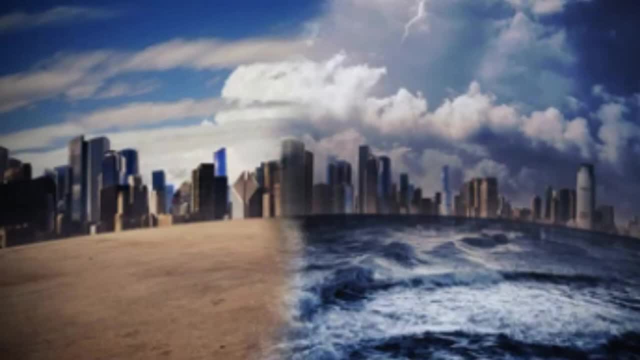 Environmental geologists work with soil scientists to understand how soil characteristics impact ecosystem health and how soil characteristics impact ecosystem health. 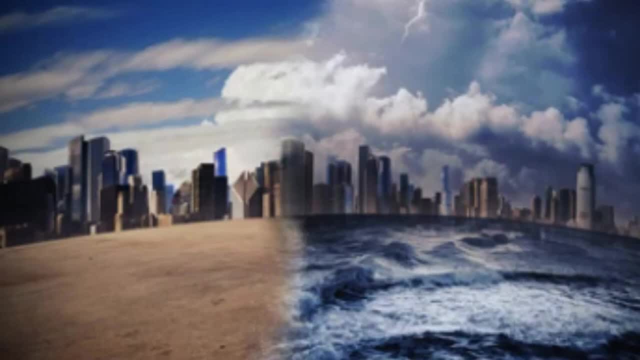 Human activities such as agriculture, mining, and construction can impact soil quality. Environmental Science 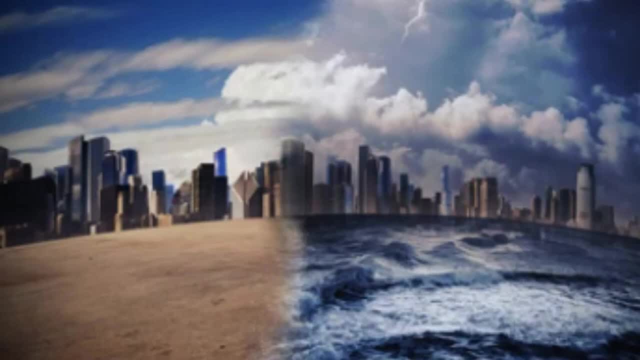 Environmental science is a broad field that encompasses the study of natural and human-induced environmental changes. Environmental geologists work closely with environmental scientists to 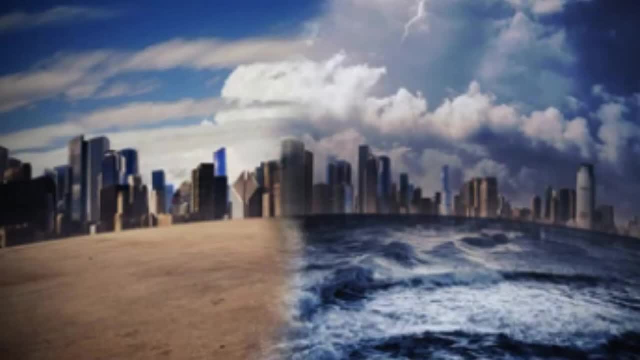 understand the complex interactions between humans and the environment and to develop strategies for mitigating environmental impacts. Ecology 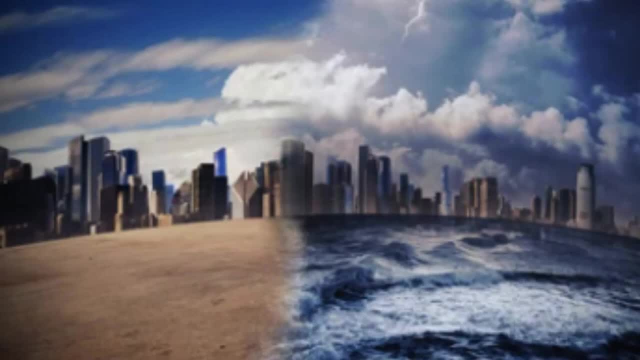 Ecology Ecology Ecology Ecology is the study of the relationships between living organisms and their environment. 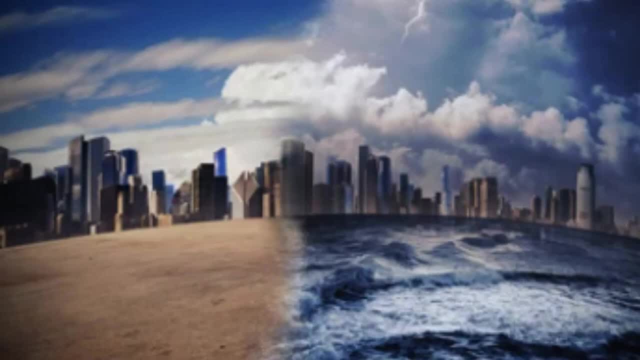 Environmental geologists work with ecologists to understand how natural systems function and how human activities can impact ecosystem health. Climate Science 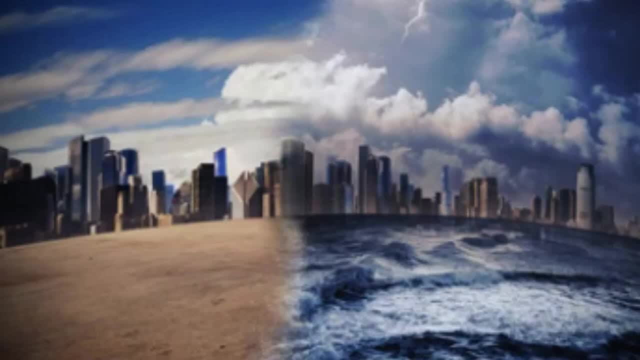 Climate science is the study of long-term patterns and trends in the Earth's climate system. Environmental geologists draw on climate science to understand how human activities are impacting the Earth's climate system. Environmental geologists environmental economy Environmentalżenia Environmental Climate Environmental Environment does not rely mainly onostat licenses, but also on the painting of Rh晚上ız' human life's size. Environmental geologists try to vocêis toiana' the impact of climate service and to develop strategies for mitigating the impacts of climate change. Geographic Information Systems- GIS-GIS is a computer-based tool that allows for the analysis and visualization of spatial data.